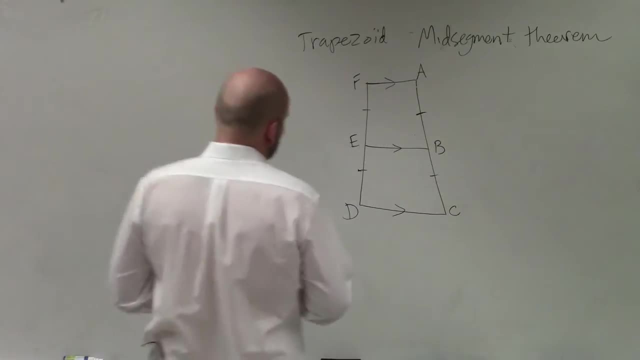 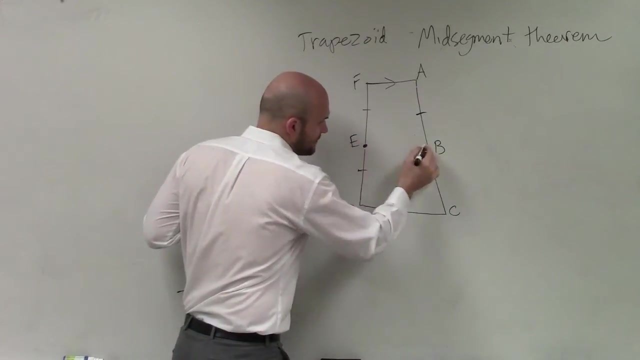 ah, here's what we have. ladies and gentlemen, if we have this trapezoid, alright, and what I want to forget about this is so we have this trapezoid and at this trapezoid, Zach, please turn that back down. okay, just face it down for this once you look up. 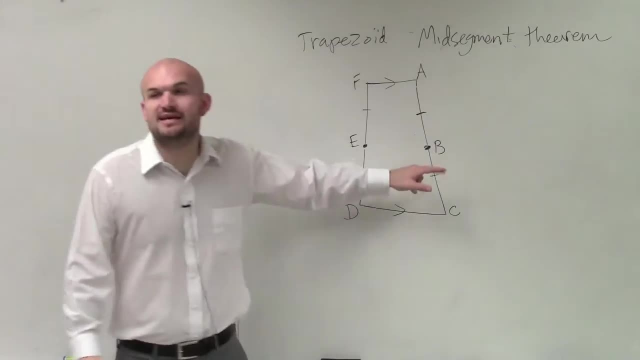 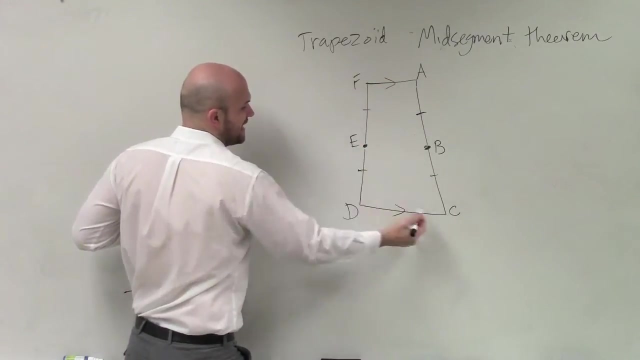 there. so if we have this trapezoid and I find the mids, if I find the midpoints of both of my two sides right now, we can see that AF and CD are both parallel lines correct, and if I determine the midpoint, that means I 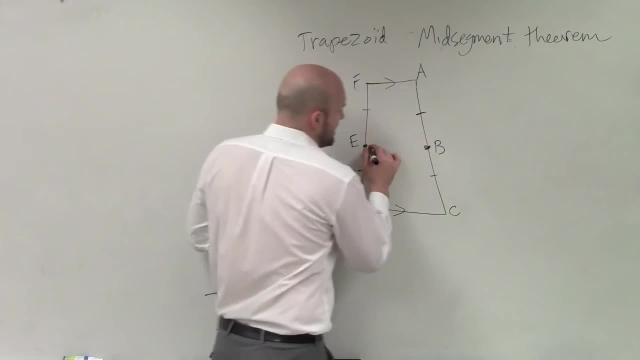 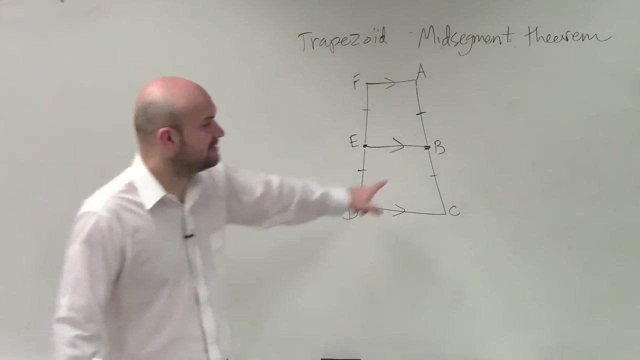 break both of those sides in half and then I draw a line that is again parallel to both those lines. then I can be able to determine the distance of this line. The way that I determine the distance of this line goes like this: 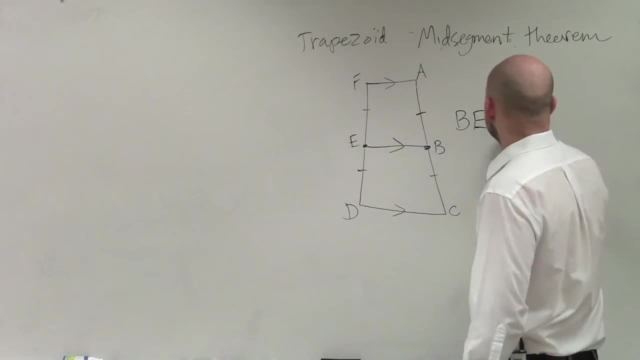 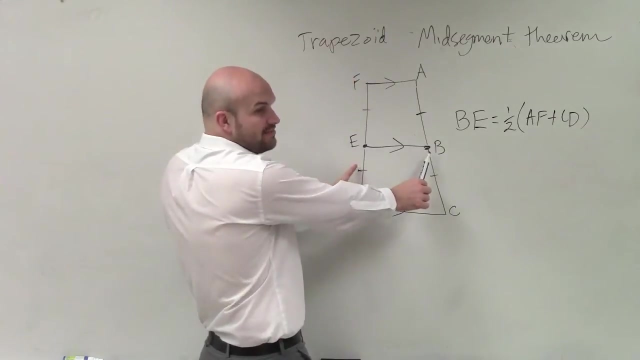 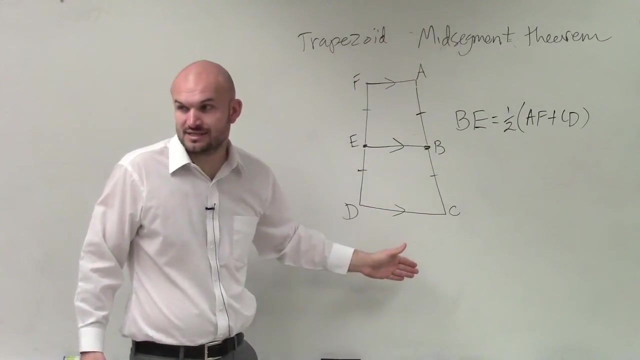 The length of BF or BE is equal to 1 half AF plus CD. So if you have a line that is parallel to your other two sides of your trapezoid and it is in the middle, then if you add the lengths of your two bases, 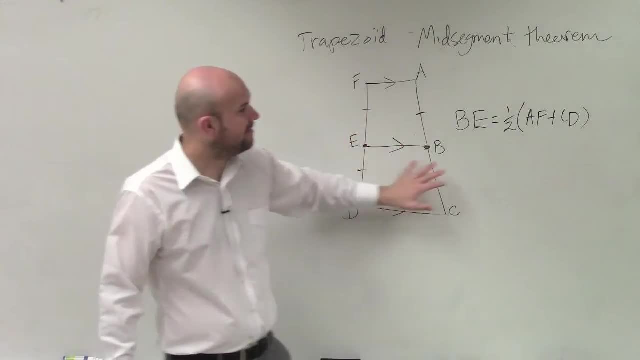 and multiply it by 1 half, or divide it by 2, whatever you think about it, then you will have the distance of the mid-segment. OK, You got it again. Absolutely, If you have a line that is parallel to your two bases. 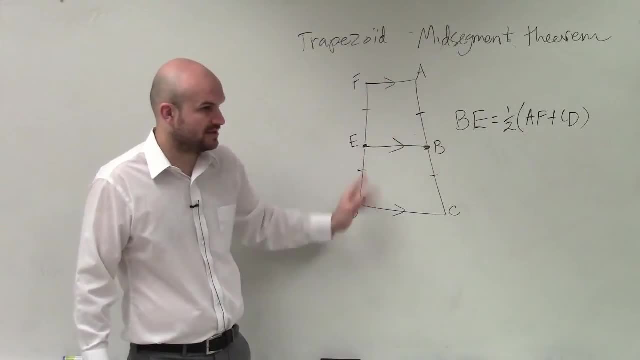 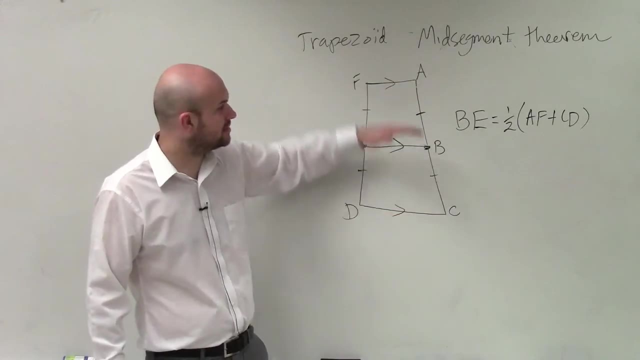 and it is in the middle between your two legs. it's in the midpoint of your two legs. then, to find the distance of that, you add the sum of the lengths of your two bases and then multiply it by 1 half and you'll.